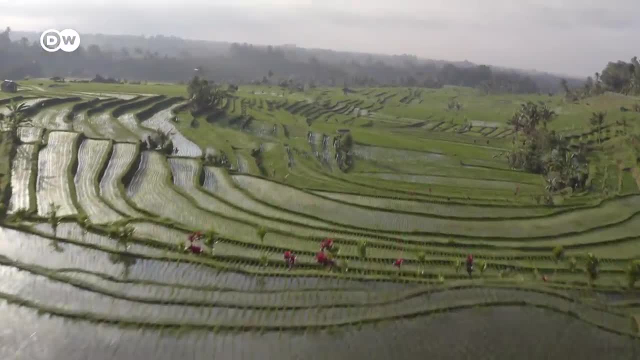 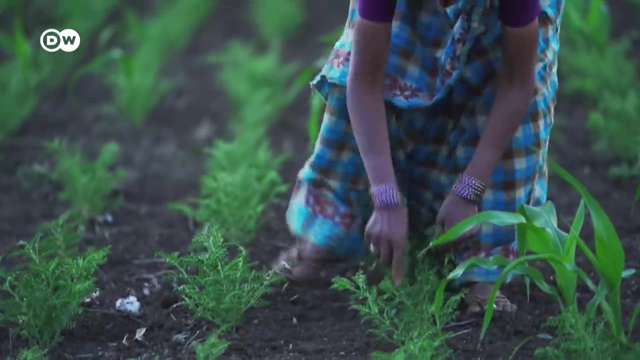 and high-yielding seeds began to be used across the global south. Some estimates say it saved over a hundred million lives in countries that were on the verge of a food crisis For a while. economies prospered as more people were fed. It seemed like a. 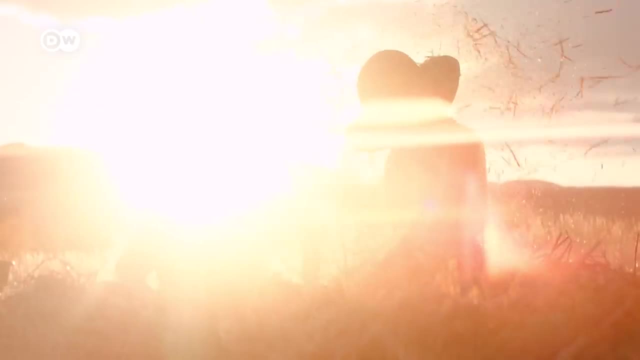 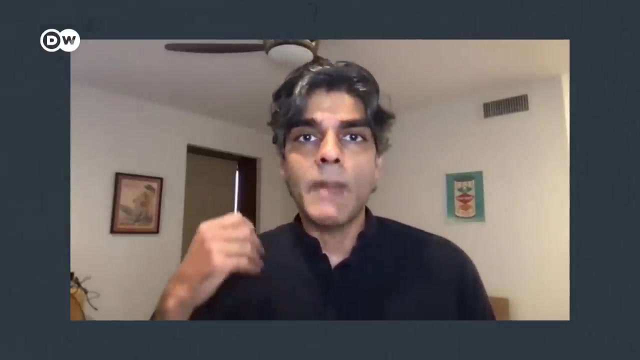 magical solution had been found. Lately, however, this method of farming has seen a lot of critics. The one thing you're not allowed to think the green revolution is is some magical chemical intervention that succeeded in feeding the world, because we've never reached that stage under. 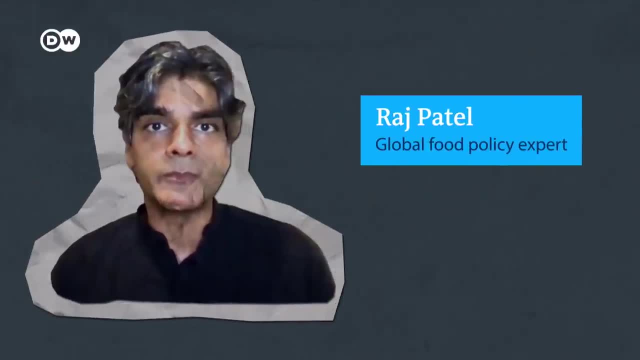 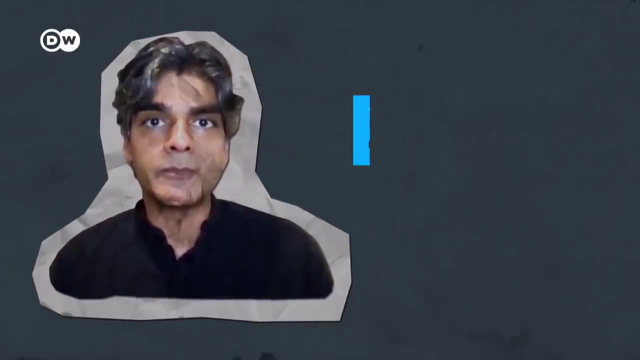 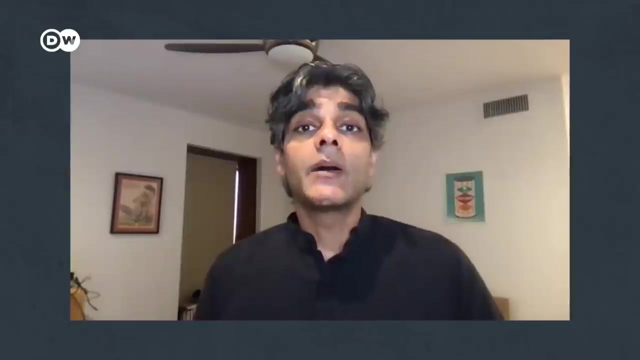 you know the past 200 years for sure. Raj Patel is a well-known food expert who believes the green revolution has caused more damage than good in the long term. Yield is getting more per unit of area of any given crop. Now you can do that by improving the genetics of the crop and then 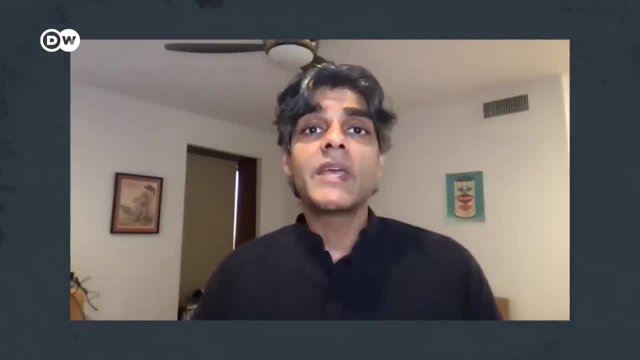 throwing chemicals at the ground, And for a while that might work. In the long term, of course, what you end up with is causing all kinds of soil chemistry problems, And so, for example, in Punjab, in India, right now, in the epicenter of the green revolution, you see. soil fertility plummeting. One intrinsic problem is the way in which pesticides work. You have this thing that is called the pesticide treadmill: The more pesticide you apply, the more you need to apply. It's almost like a junkie. You get addicted to it. no, The more you take, the more, the less effective it becomes. 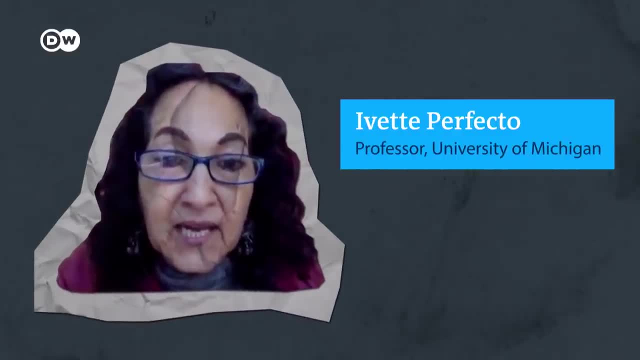 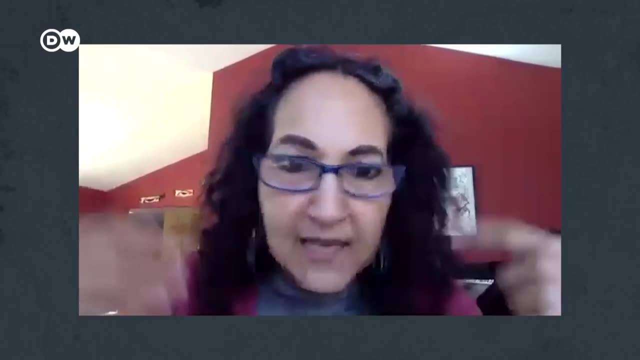 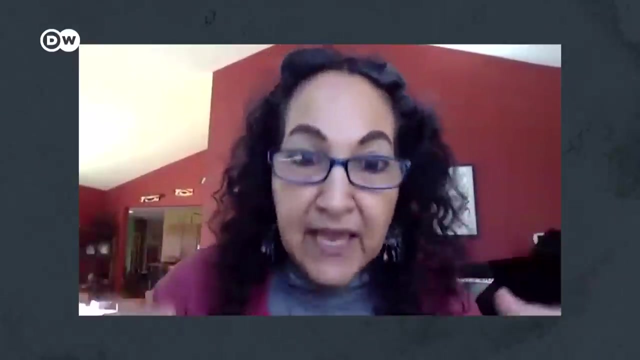 and the more you need to apply. Yvette Perfecto has spent her career studying herbivores and pests and how they react and respond to pesticides. It's like us evolving resistant to an antibiotic. no, If you know they are effective to some. extent, but then eventually, especially if you abuse them, then you evolve resistant to them. The same thing happens with insects: They evolve resistance to the pesticides. So the more you apply, the more resistant the population becomes and the less effective the pesticide becomes. Coating the soil indiscriminately also leads to other 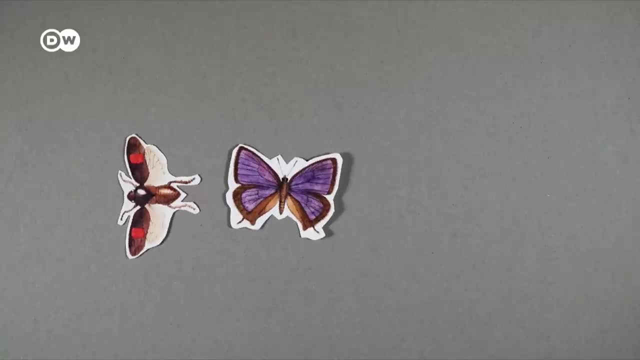 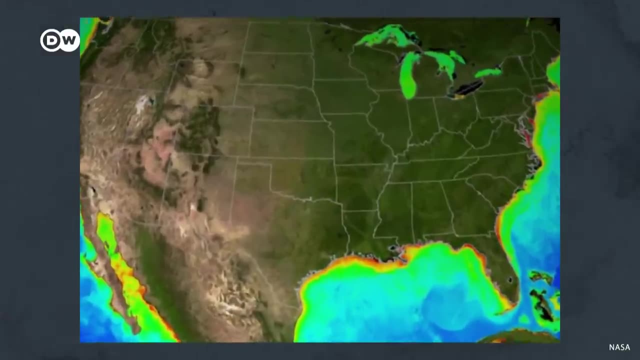 species dying off. In the last 30 years, global insect populations around farms have declined, declined by up to 75 per cent. And that's not all. Runoffs from farms fill rivers with chemicals and when they drain into the ocean, they kill. 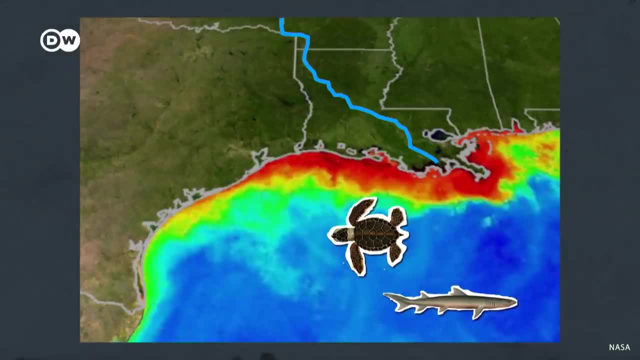 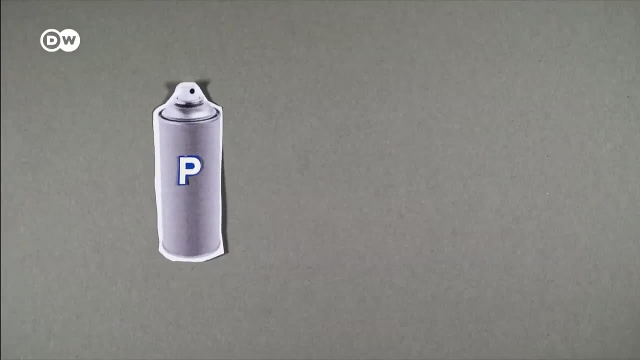 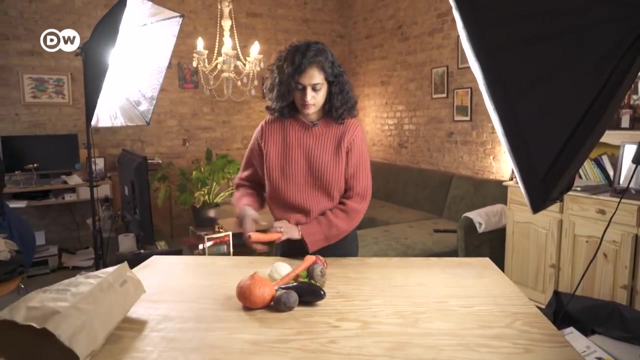 off large populations of wildlife, from sharks to turtles and whales, like in the Gulf of Mexico's Dead Zone. Not to mention that spraying pesticides also causes farmers problems from skin rashes to long-term lung damage, And the residues that remain on produce can cause long-term health conditions. among the 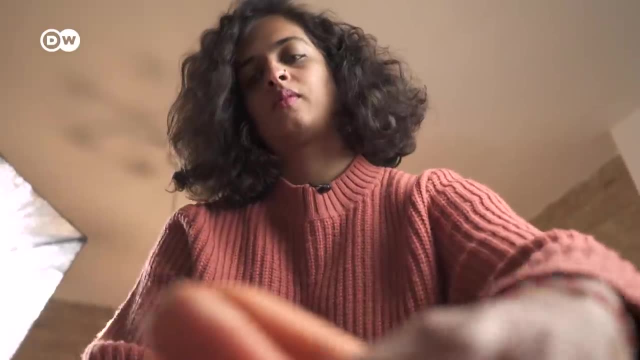 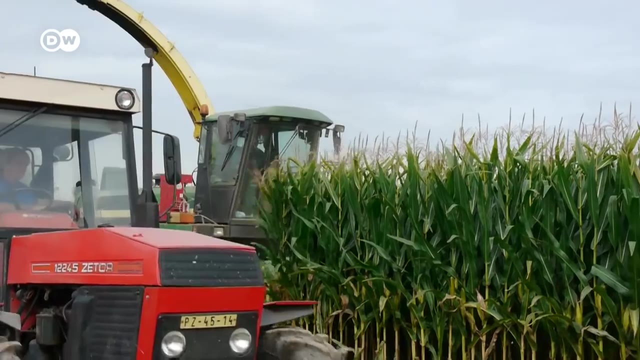 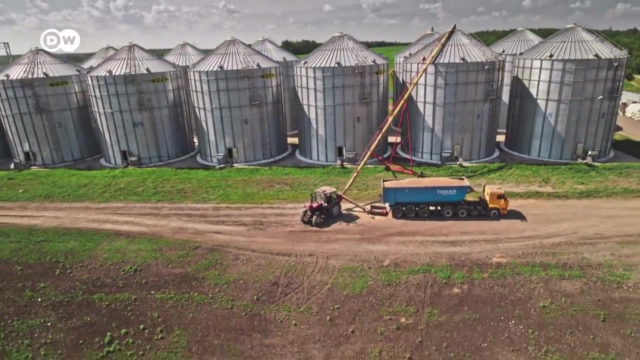 people that eat the fruits and vegetables. That's a lot of negatives, But proponents of industrial farming say alternatives are either too expensive to scale worldwide or use too much land, Especially as our remaining forests need protection now more than ever. But is this still true? 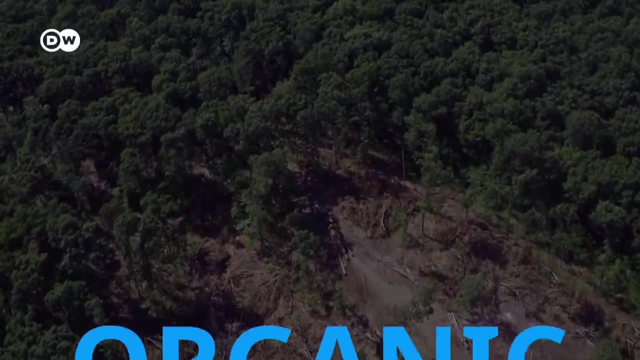 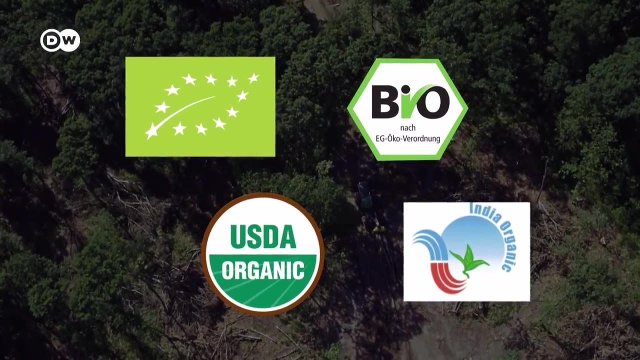 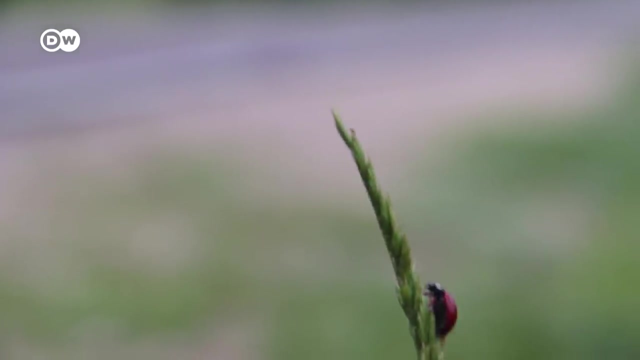 Organic is the umbrella term for anything grown without chemical pesticides. Regulation for what is and isn't organic is not Organic vary by country, but generally fall in line with natural biological systems and protecting water, soil, air and biodiversity. Organic farming methods can include introducing natural predators to keep pests away or growing. 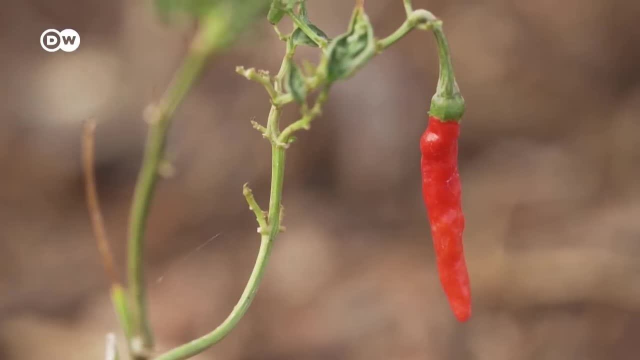 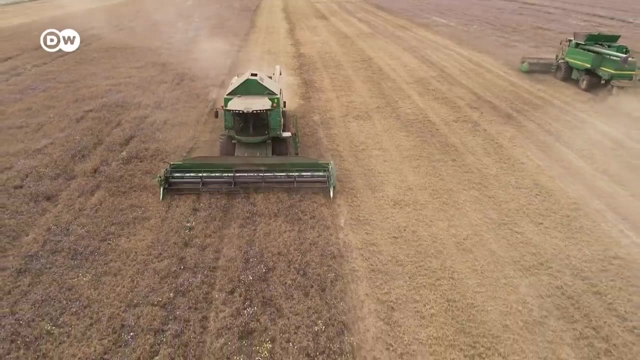 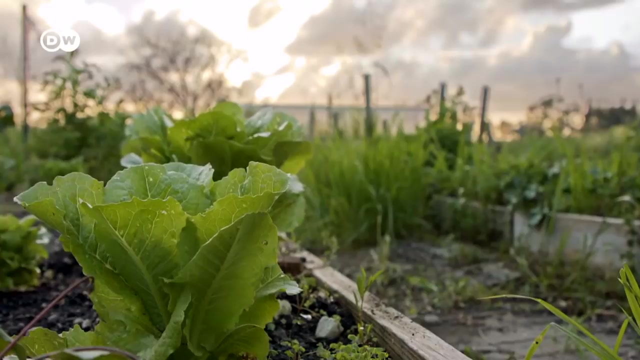 multiple crops to improve soil health, and even using organic pesticides that are generally less toxic than chemicals. This does lead to more land needed for agriculture and less yield overall. The jury is still out on whether organic food is actually much more nutritious, But what is certain is that organic vegetables contain far fewer pesticide residues and are 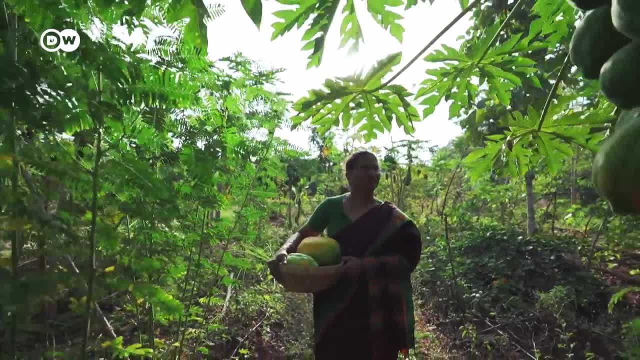 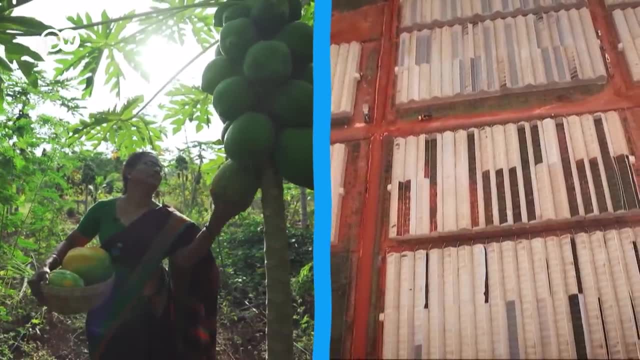 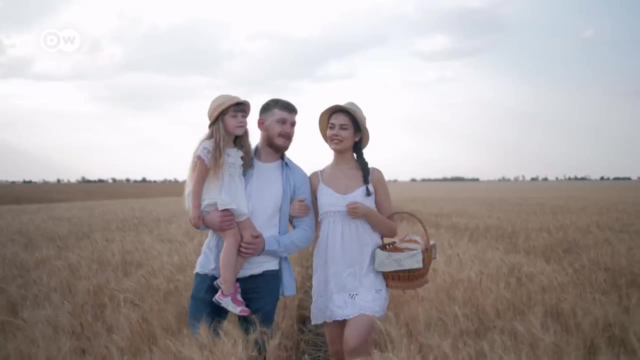 therefore healthier. But there are a lot of grey areas. Organic farms can be small scale and cater to local communities, or they can be large and industrial, transporting food over large distances, sometimes overseas. So not all organic farms mean local and happy and pure. 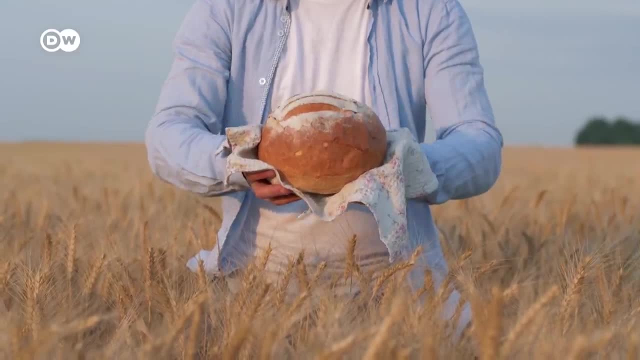 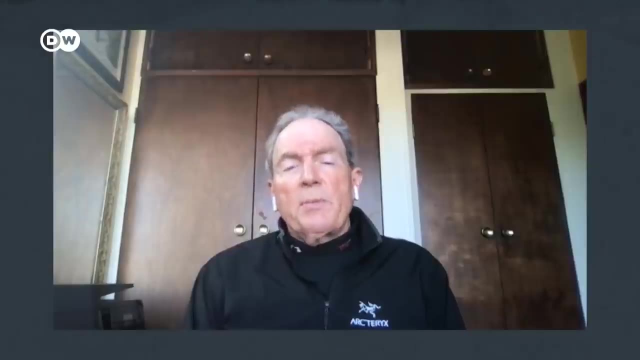 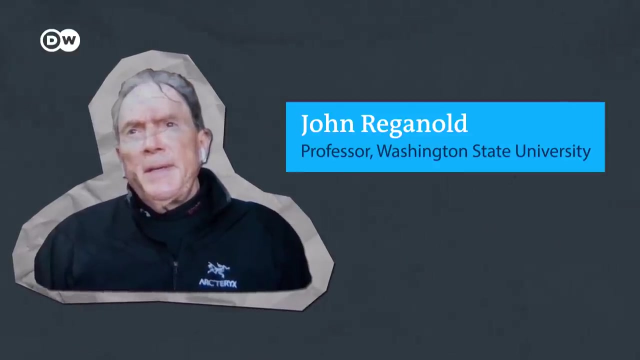 Organic farms can be large and industrial, transporting food over large distances, sometimes overseas, With so many ifs and buts. how do the two compare? We had looked at 40 years of all the studies done comparing organic with conventional farming. Reginald and his team found that while conventional farms produce 10-20% higher yields, organic farming is not only better for the environment but, and most surprisingly, It was more profitable. significantly so, And part of that reason is because organic farmers get a premium for their food. They get more money for their food. Over that 40-year period between 1975 and 2015,, the premium averaged about 30% more. 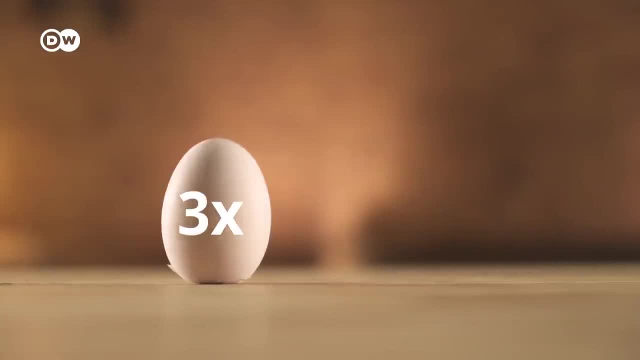 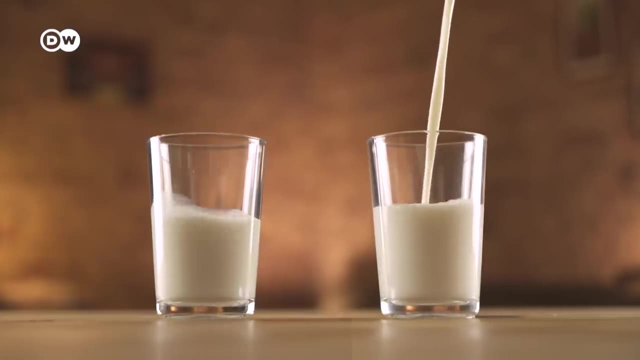 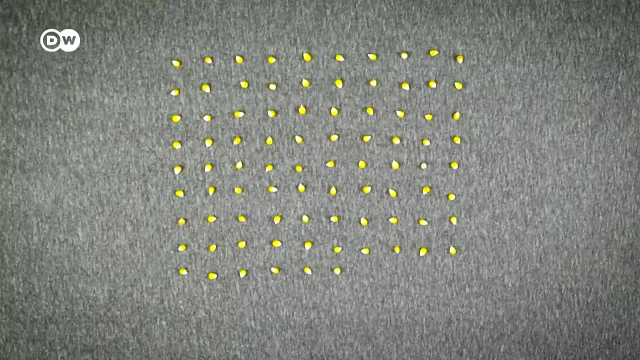 This high price of organic food can't be ignored, though. Eggs cost up to three times more. in Germany, where I live, for example, Organic milk is double the cost of conventional milk. But at the moment, of all the farmland around the world, the share of completely organic 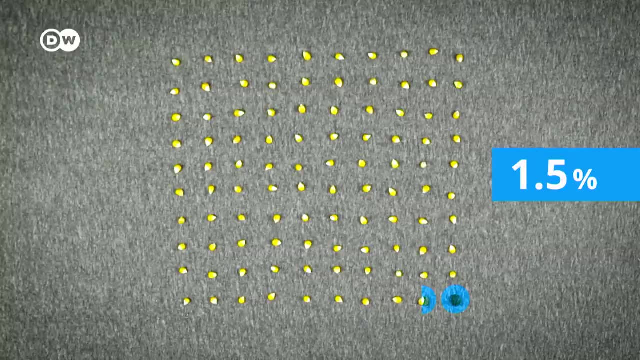 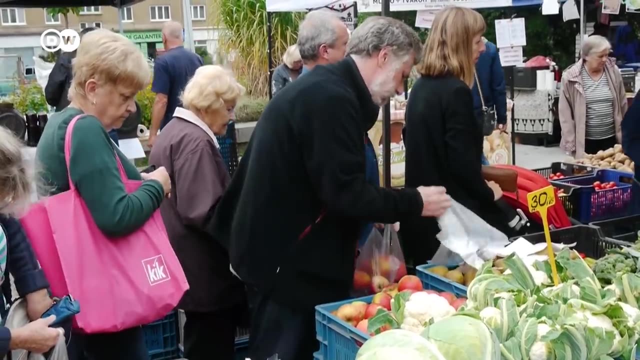 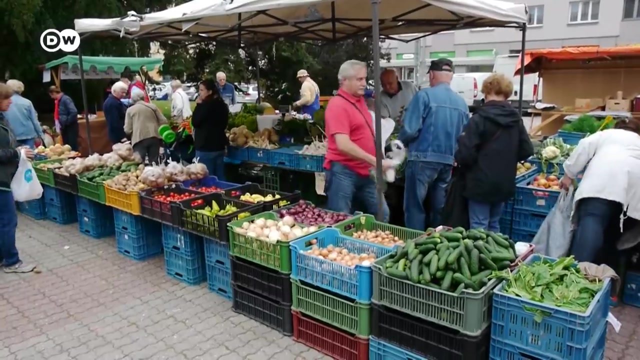 farms is just 1.5%. As this grows, the price of organic produce is expected to fall to make organic food more accessible. In fact, prices have already largely started to fall in the last 10 years around the world. But do we need to cut down more farms? 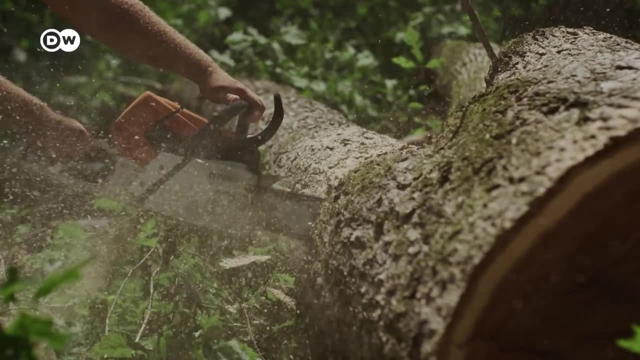 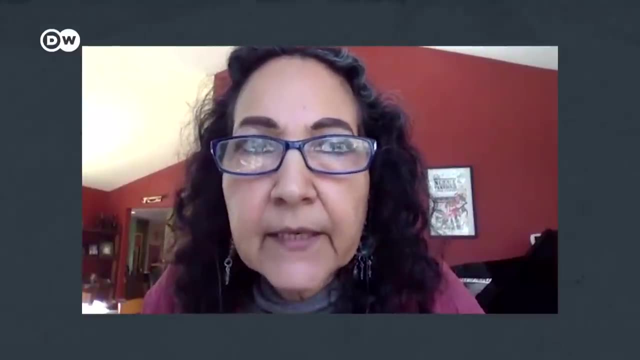 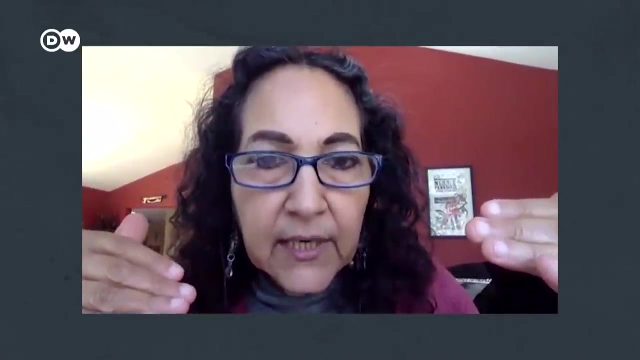 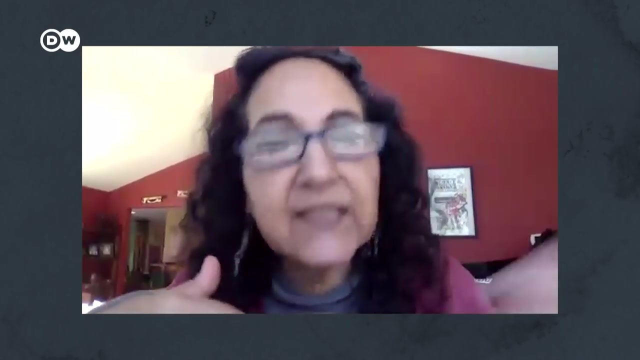 Forests, Or can organic yields sustain the world? Our studies show very convincingly that, given the yields that are produced in organic agriculture and the amount of food that is needed to satisfy the nutritional requirement of the human population, that it is possible with organic agriculture to produce enough food to feed people. 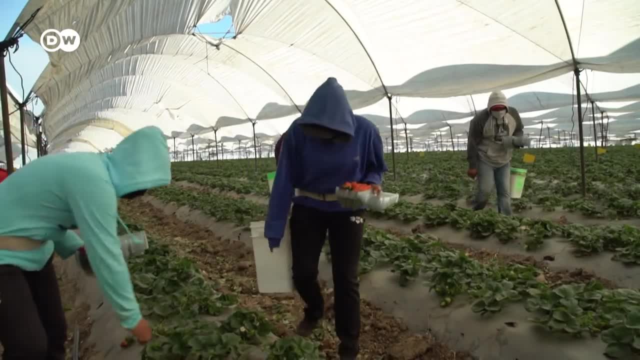 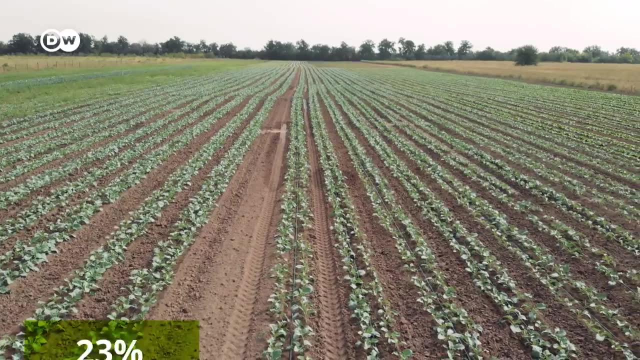 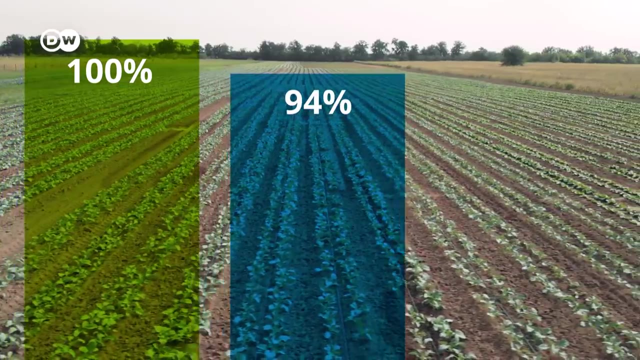 Many other studies have come to the same conclusion, But with one major caveat – our diets. If people ate only vegan food, 100% of the population could be fed on organics, using just the land we already farm on. Vegetarianism would give this a 94% success rate and a Western-style meat-heavy diet. gives this a 15% chance. There is another big factor as well – inefficiency. Right Right now, a third of all the food we produce worldwide gets wasted, And we also basically produce a lot of I wouldn't call it food, but there's a lot. 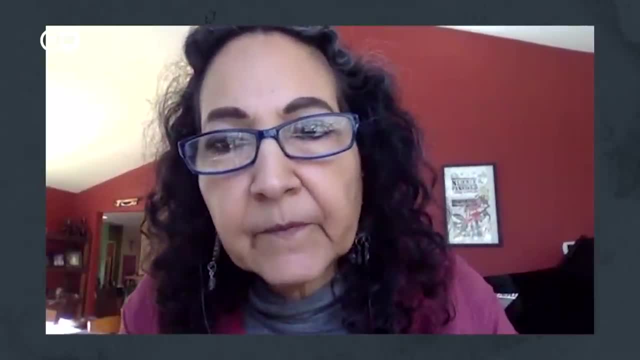 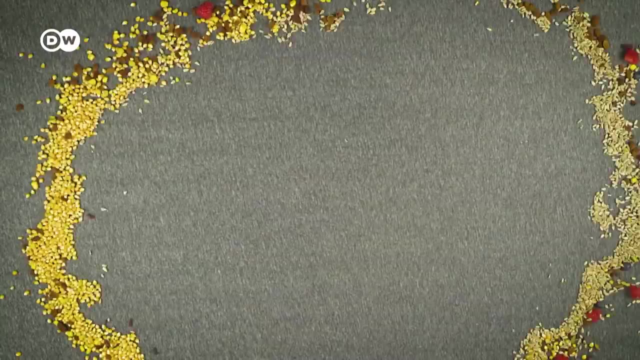 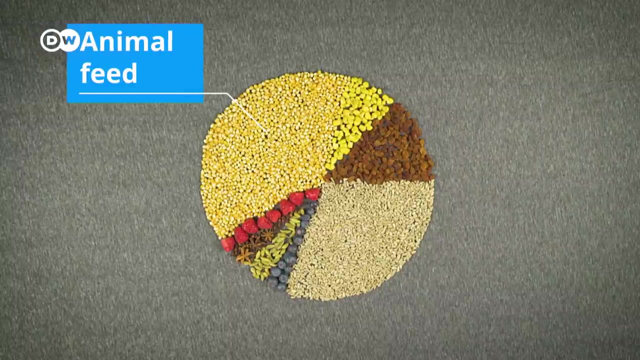 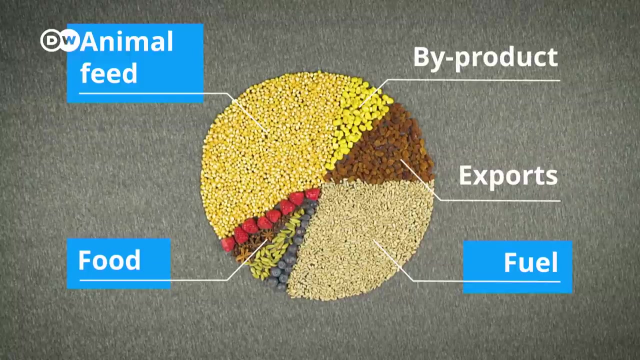 of grain that's produced to feed cars, for ethanol or biofuels. A good example of inefficiency of land use is corn. Most corn harvested in the US goes directly to feed animals or to be burned as fuel, while less than a tenth enters the food system. 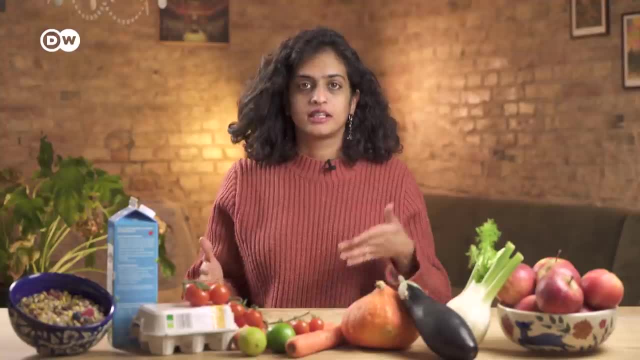 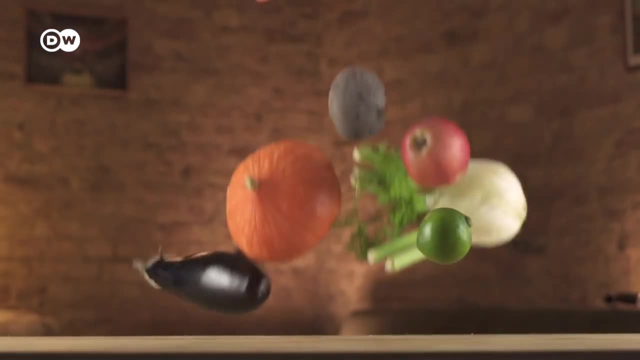 So, in theory, we could feed the world with just organic food, especially with a more plant-based diet and more efficient farming systems. But do we need to get rid of all pesticides? Maybe we don't need to be so radical, And it might be. we live with…. 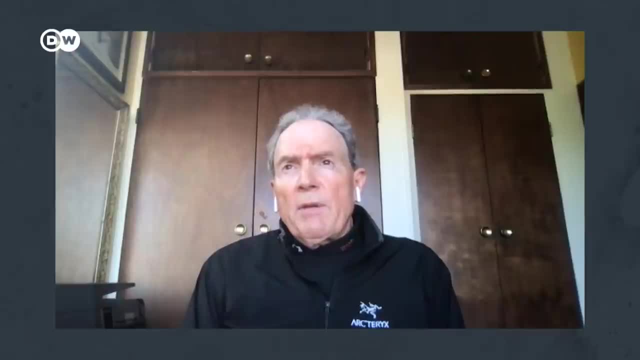 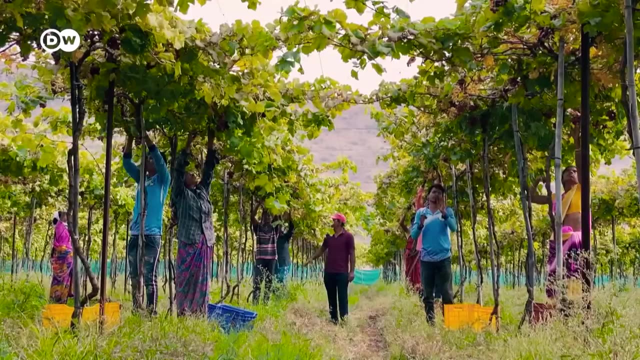 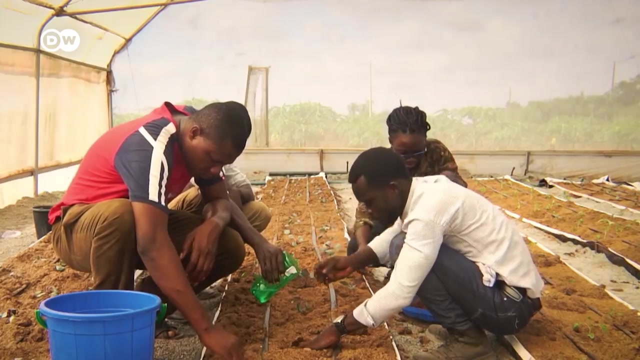 We live with… Some of these synthetic chemicals, but we use them just to tweak. We use them in very small amounts. We use them more as a last resort. Around the world, more and more farmers are integrating their farms growing organic crops.